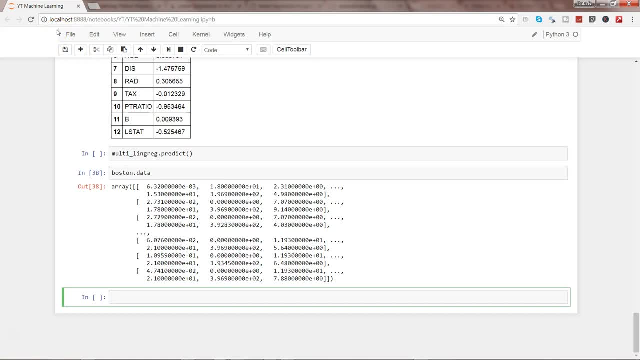 Hey guys, this is Abhishek, and in this video I will talk about how you can split the data for the better model building. So what I mean by splitting the data is that as well, a part of the standard statistical model building process, you want to reserve some data for the validation of. 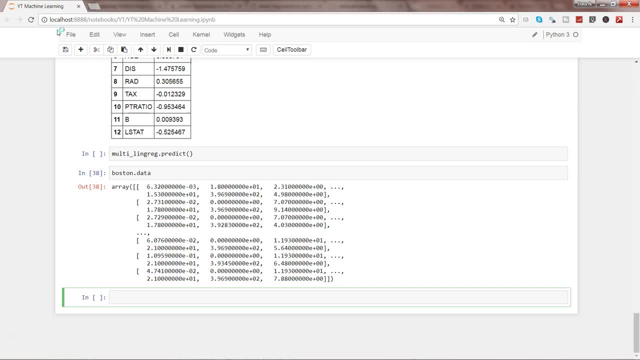 prediction model That is really required to test how much variance is there in your predicted and observed value or test values. so what we do is generally, as a rule of thumb, we reserve 70 of the data in the training set and rest other 30 percent on the testing set. 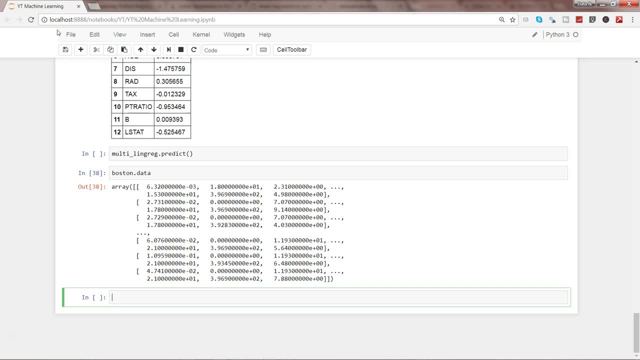 with the help of the training data, we produce the model to be. basically, we say we are training the model and with the help of the test data, we are testing the model to see whether the model is performing fine or not. and this testing happens with the help. 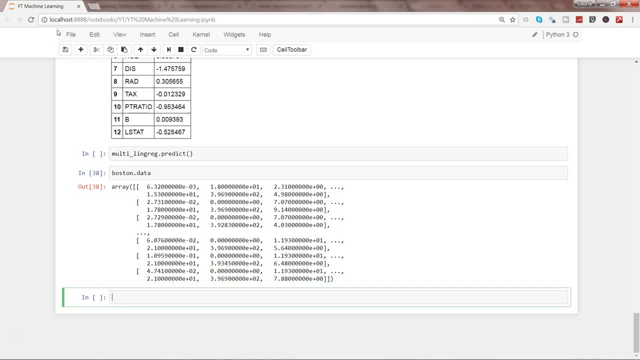 of the calculation of error matrix like mean, standard error, msc or rmsc, root mean, squared error, which basically tells us whether we are doing it good or not, and in next a couple of minutes i will show you how you can really achieve to that level. all right, so first thing is we need to 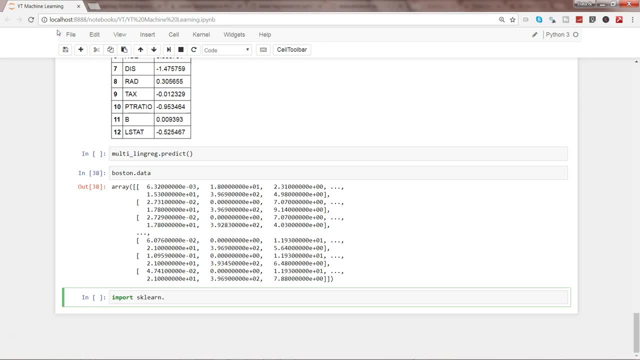 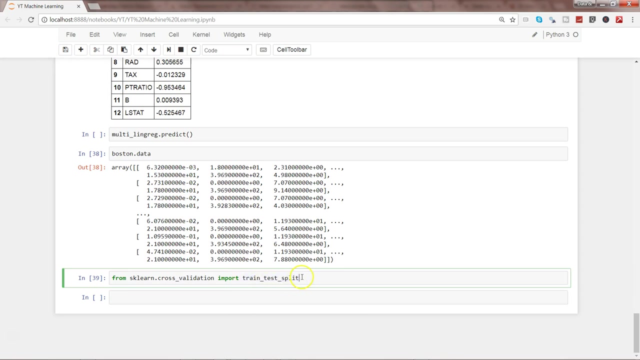 import from sklearn from sklearn dot cross c r o double s cross validation need to write from and then we need to write import import train test split. okay, so what this function does, or this this basically method does, is split the data into a training and testing. straightforward, okay, and how we specify it is basically x underscore train and then x underscore. 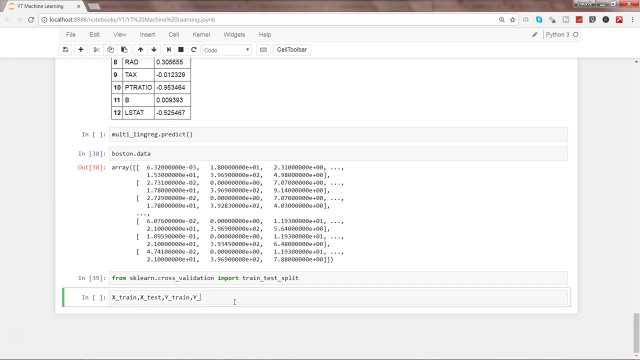 test y underscore train and then y underscore test. after that mention the train test split and then the data set name. the data is basically our boston dot data and then the price, the target variable boston dot target, and then the test size. so you have the option of specifying the training size or the, the testing size. 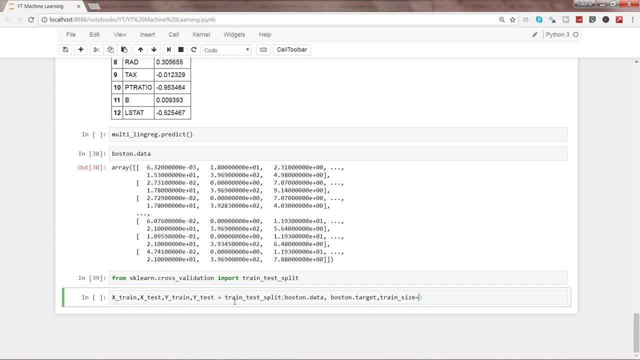 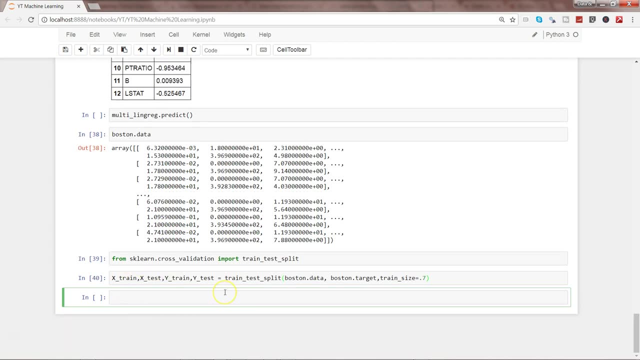 so that is, size is equals to 0.7. okay, let's go ahead and execute it. and now we have x train x test, y train, y test. what we can do is we can print the shapes of these: x underscore train dot shape, comma, x underscore test dot shape, y underscore train dot shape and then y underscore test dot. 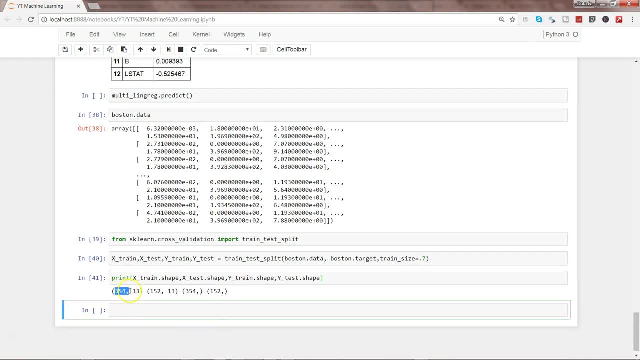 shape. so here we have three fifty four variable, uh, three, fifty four rows, thirteen variables. then in test you have one fifty two rows and thirteen variable. and then in y you have three, fifty four rows and in test you have one fifty two. so there you can see that these are evenly split. 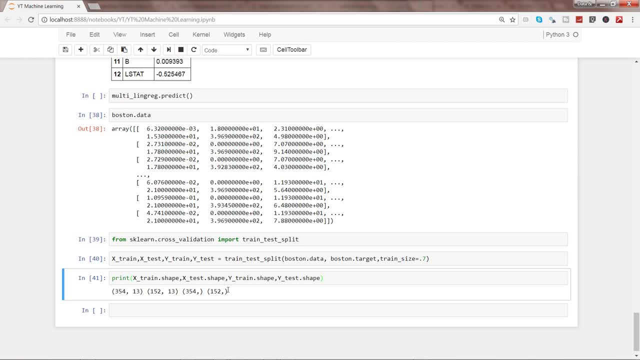 so that you don't have to manually go and use the loc, illc or numpy array- related uh, you know- functions or slicing andиcing. so this is pretty handy. and you can specify train size. you can specify even test in the score size. you can specify even test in the score size. you can specify even test underscore size. 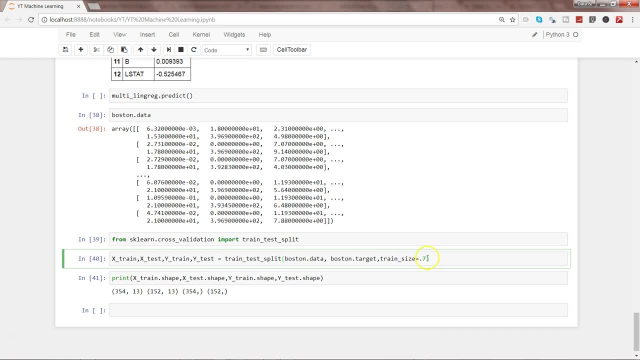 If you want to look more in-depth into it, you can press. you can be there in the function and press Shift-Tab-Tab. let me just close this Shift-Tab-Tab and then you have different parameters. so, for example, test size, train size is the one that we used, couple of others. 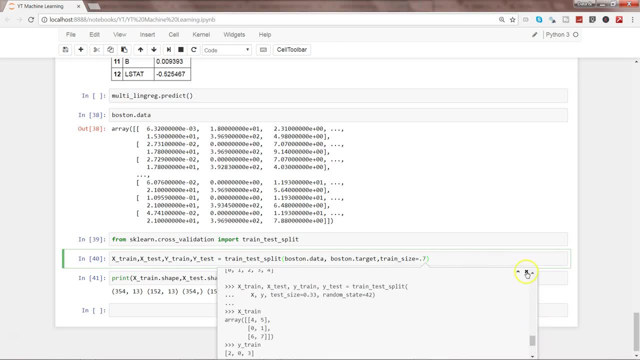 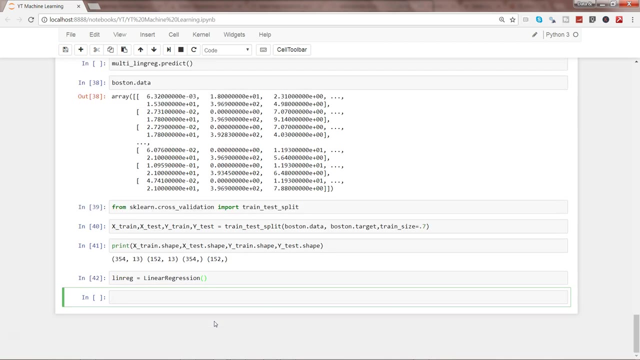 which you can further explore. alright, I'll just close that And after that I will simply initialize the linear regression again and execute it. After that I will say the linrackfit and we will say: we will take the training dataset. 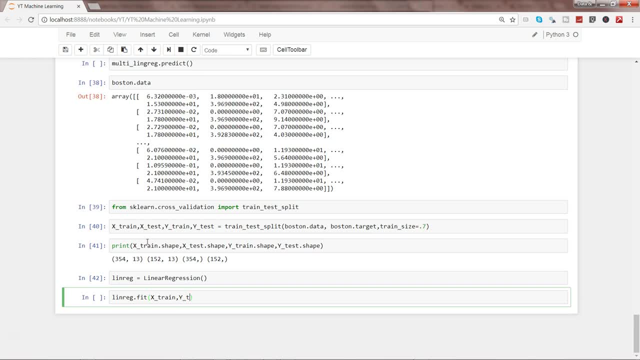 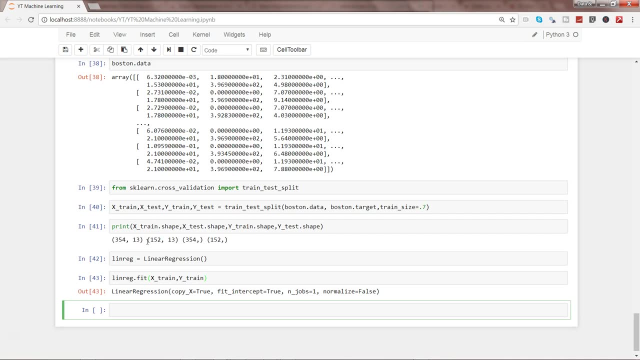 and training is our x underscore train and then y underscore train. execute it and then we will. We have already fit the value with the help of x train and y train and after that, in the previous video, if you have seen, we have gone ahead and predicted the value with the. 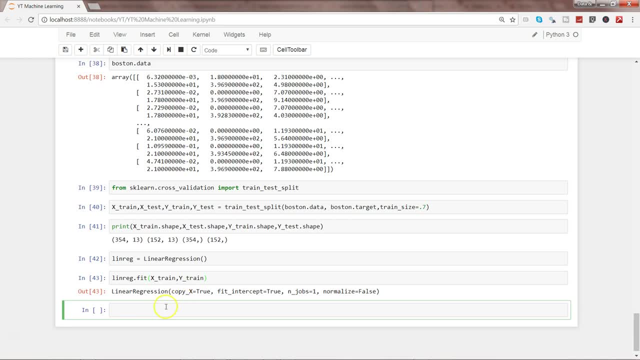 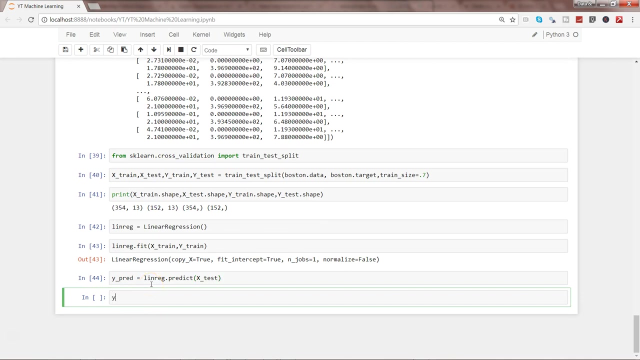 help of the predict method. But now for prediction of the value, what we have is the test dataset. So what we will say is y underscore pred, which is basically predicted value. linrackpredict specify x underscore test. Now we have the y predicted value based on that validation dataset that we had. 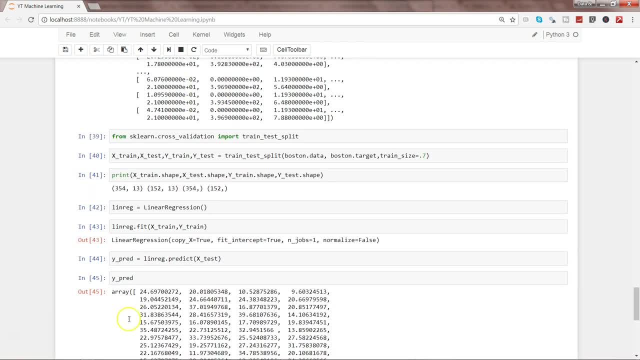 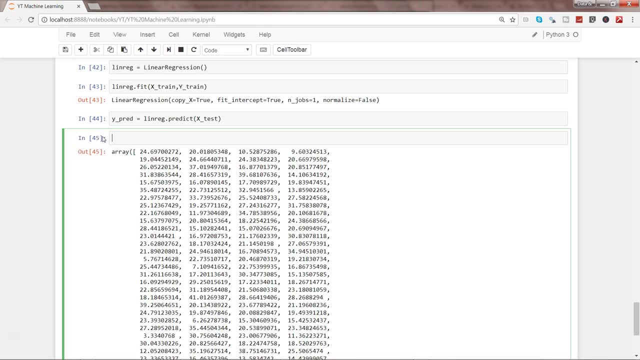 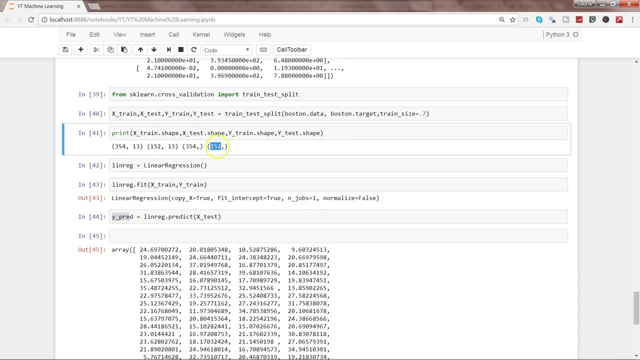 So y underscore pred. if I write, and this is here, all these predicted values, Now we want to calculate the errors. right, because we have the predicted values and, similar to the predicted values, I have the test values, y test values, which both can be compared because, if you see, 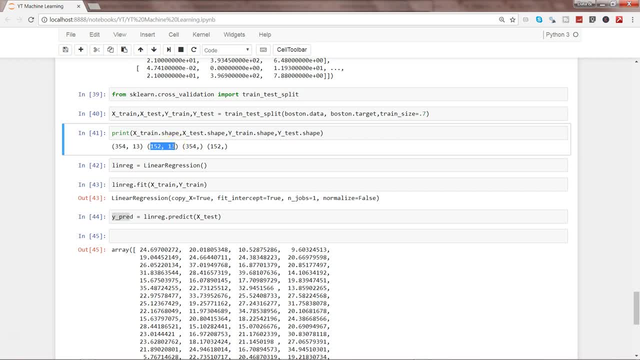 in the x test dataset, which we want to test it against, the model has 152 rows, So the output- predicted value output- will have the 152 rows. Similarly, in the y test you have 152 rows, So that's more of an apple to apple comparison because we have already split the data properly. 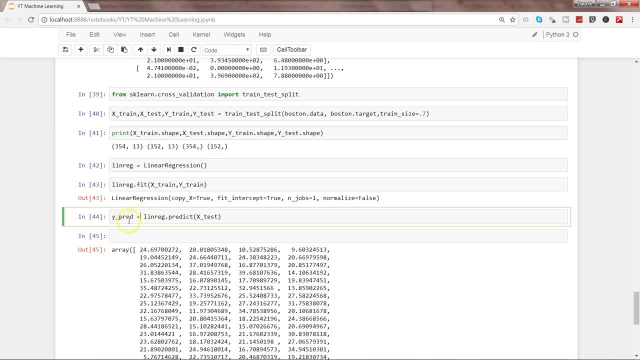 so if y is given, that is the required shape. So once we have this, what we can do is we can use np, dot mean, and then what we have is the predicted and test. So we will write y underscore test minus y underscore pred. 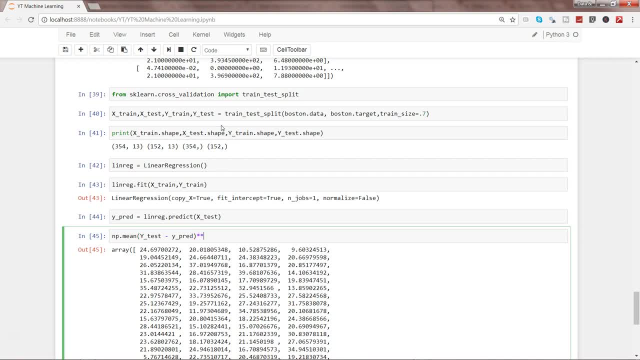 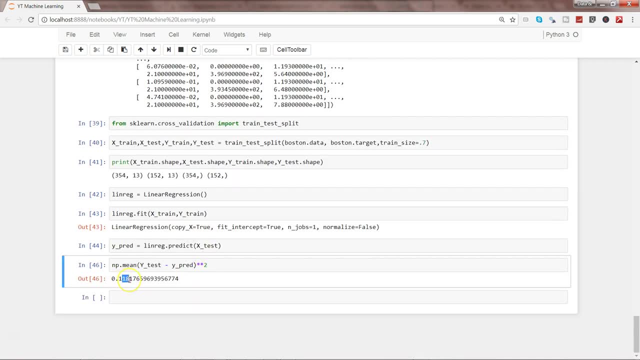 Right And then, since it is a square Right, will write the square function and let's go ahead and execute it. so what we get is is basically 0.118 right. so this is one way of going ahead and identifying the mean squared error. so i will. 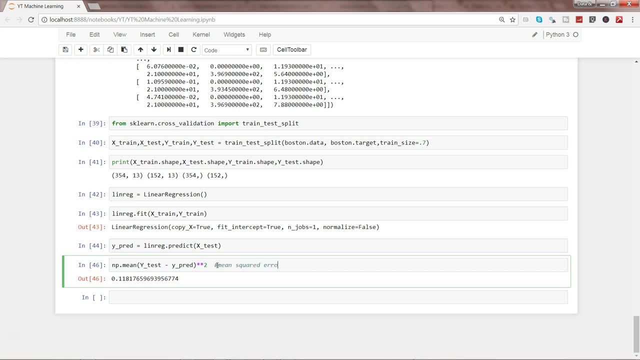 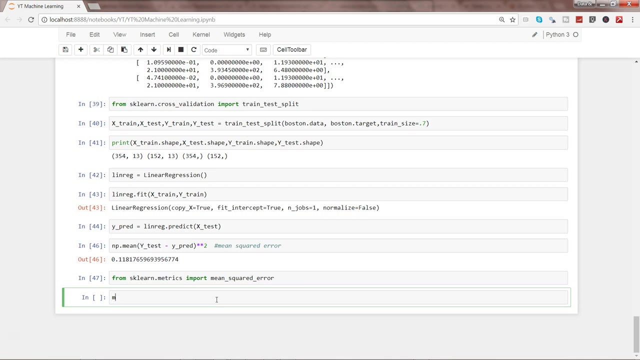 just write mean squared error. if i want i can. from sklearn dot matrix i can import mean squared error and if i execute it, i will simply go ahead and write mean squared error within the function. if you can see, y underscore true is nothing but y underscore test, which is: 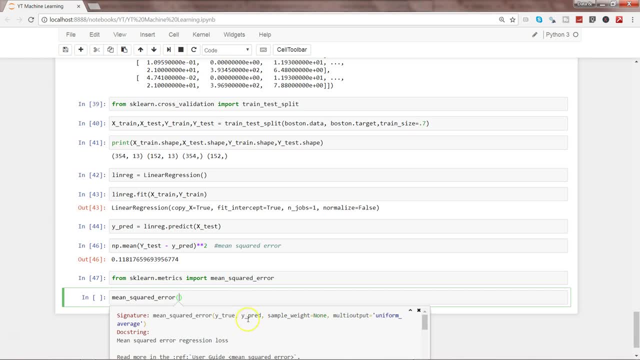 the true values and then y underscore right is basically the two main uh out, two main parameters you need to provide. so let's go ahead and see whether we get the result similar to this y underscore test, because these are the true values, and then y underscore thread and go in. 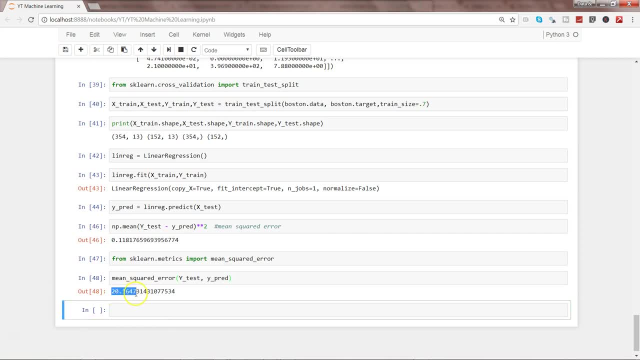 and execute it. so in this case it has come 20.. ideally it should be similar to this, so i think i have done something wrong over here. so what we are saying is: so squared is necessary to to basically, you know, get the positive values in case if you are getting the negative value. 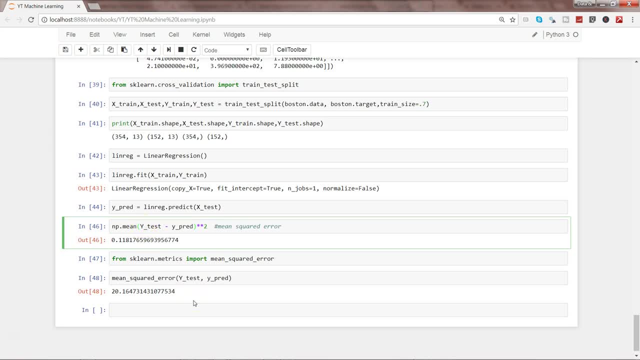 so i think what is required is is another or over here the break and then end it over here. all right, so if i go ahead and execute it, yeah, so now it is coming. so that's the thing i got over there. that's why i was wondering why these two things are different. ideally, 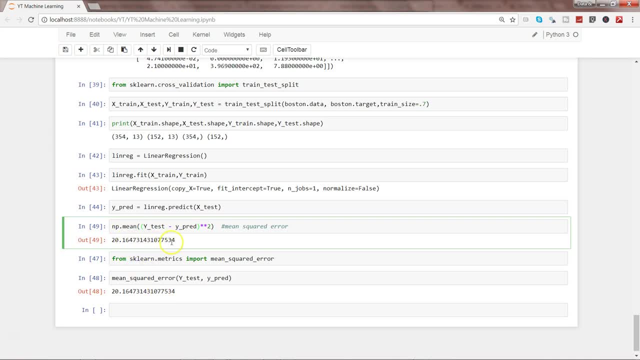 they should be similar. so if you look at, even up till the 10th or 12th decimal point, the values are same. so that's the manual way and, as you can see, you can sometimes incur error. so you have the direct function, which is a mean squared error, and with that you can get the mean. 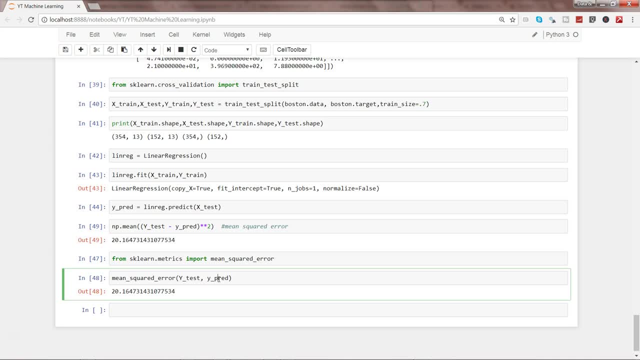 squared error. now the interpretation is bit difficult because, if you look at, it's basically a difference between the line of regression and your actual value. so line of regression represents represents basically the outcome based on your prediction and then your actual values basically represents your actual y value. So what is the difference between that? We are calculating that. 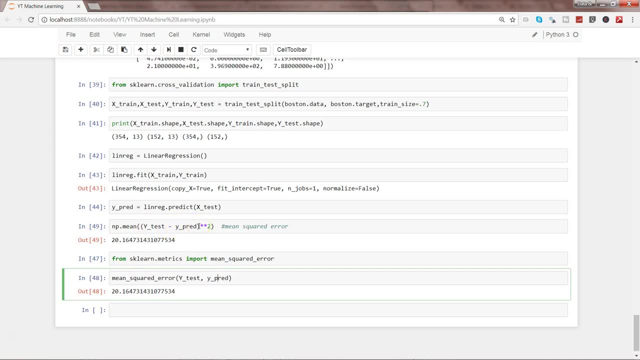 as you can see. and then we are squaring it, because the requirement for the mean squared error that it should be positive. So we are squaring the negative values and then it is converting into a positive and the final output is basically 20.164731.. Now how you can use it for further. 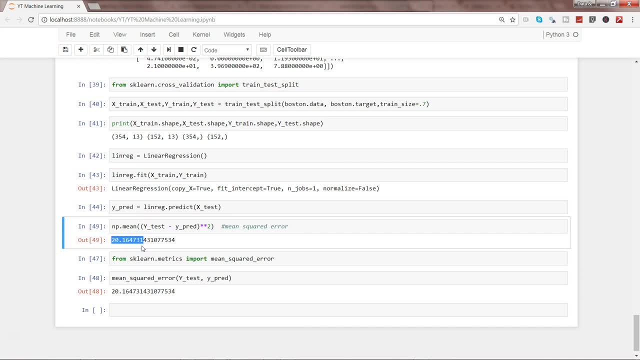 evaluation is that. let's say you are experimenting it with multiple variables Here. you know we have just gone ahead and taken the entire data. but let's say you are saying, okay, I want to, based on your business knowledge, you want to select only certain value or specific variables. let's say out: 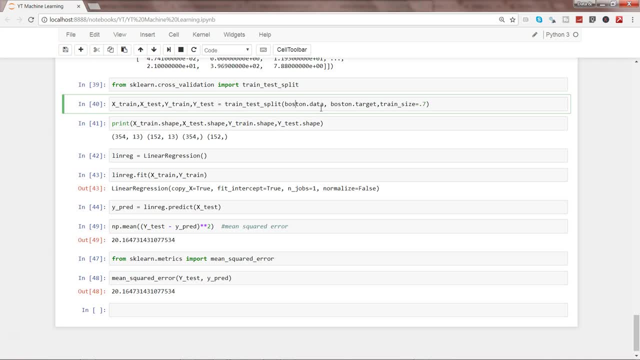 of 12 or 13 variables. you want to select 5. variables and want to see, and then you experiment. then you probably did some exploratory data analysis and you saw, okay, couple of other variables are also showing something significant. then you can hit those variables and then see whether the mean squared. 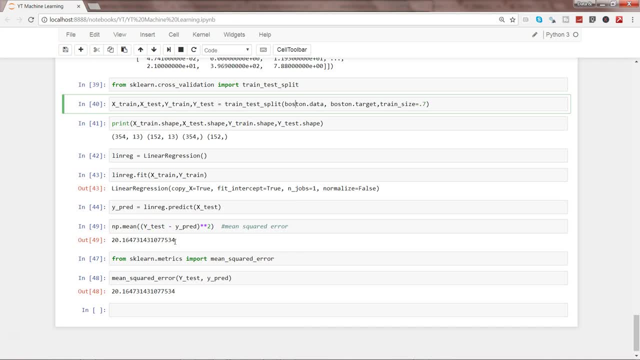 what is the value of mean squared error. So the lesser the mean squared error, the better will be the model is because this will indicate that if it is closer to the zero or if it is less compared to the multiple mean squared error based on your multiple models, then 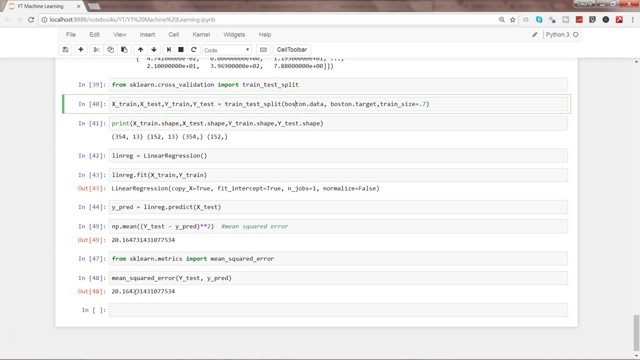 you will choose the lesser one or the one which has the smallest value, because it represents that whatever variables that you have chosen is best representing your line of regression line fit. So that's about how you can use it. You can read its documentation on the Wikipedia or there are a. 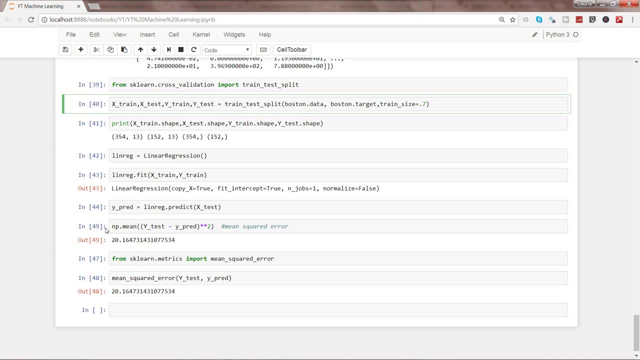 couple of other sites Which have given a good basic explanation, but basic idea. you can keep in mind that wherever, whenever the value is less based on the multiple model evaluation, you can pick the lowest one. but that's not the only thing you have. apart from MSE, you have RMSE, which is nothing but the square root. So what it does is of this value it takes the square.